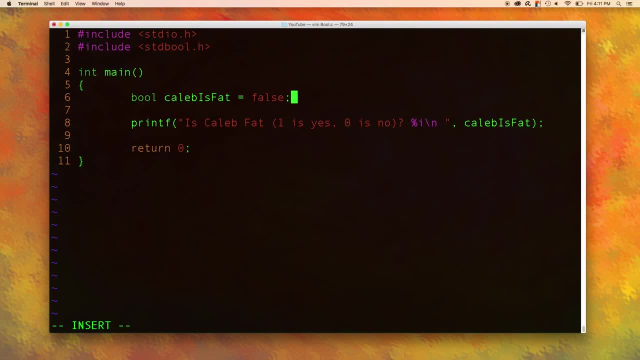 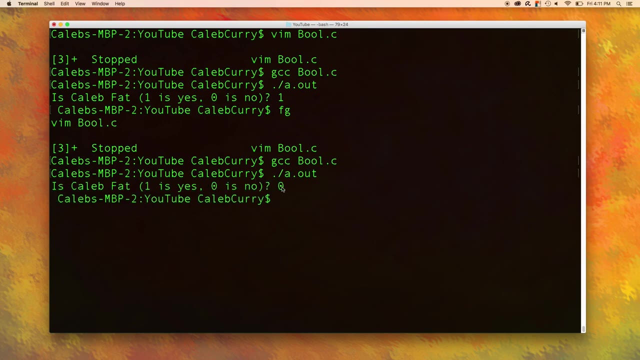 different than underscore capital bool. it just makes it easier to work with. in fact, the values stored are still 0 or 1.. so we should be able to run this just the same. let's write it and we'll compile and output it. and the output is 0 because i set it to false. but we can do more with this. 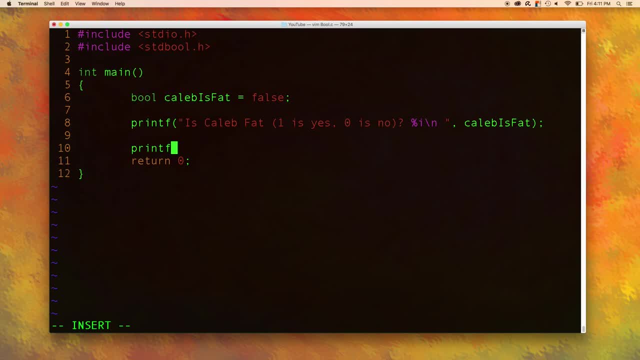 for example, if you come down here, you can put something like this: where in quotes we are going to output an integer and then go to a new line and the integer we want to output is actually caleb is fat plus 10, and that seems really, really odd. but what i just want to show to you is that there is a direct 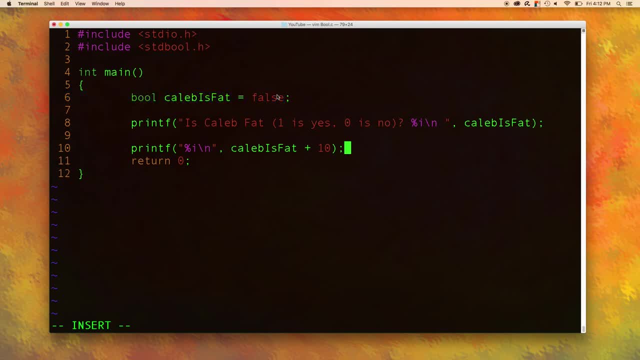 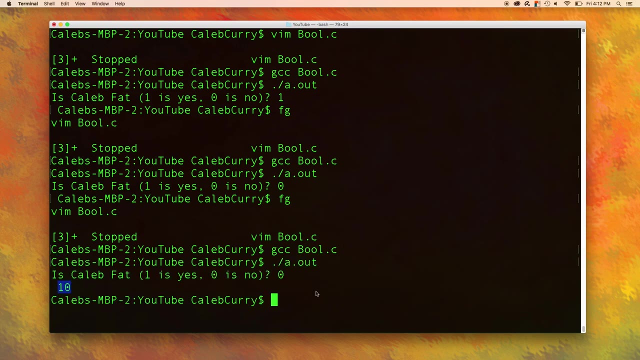 correlation between this and a number. false is 0, true is 1.. when would you actually do this? i'm not too sure, but just follow along. let's save this and run it and you can see down at the bottom it outputs 10.. just to show that it's working, let's set it to true and make sure the output is 11.. 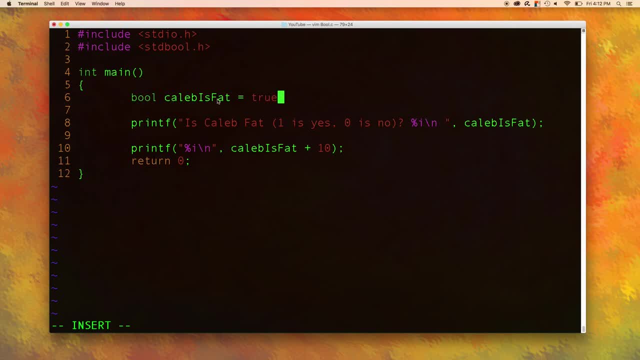 so when i change this to true, caleb is fat now has the value 1, so when we get down here it should be 1 plus 10, which equals 11.. so let's try it and you can see the output is 11.. if you're. 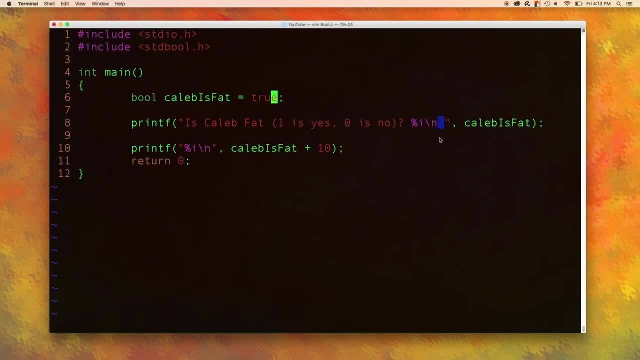 wondering where the extra space is coming from. it's right here. now there is not a format character to print out the word true or false, but later on, when we start talking about conditionals, there are ways where we could output: caleb is fat or caleb is not fat, depending on the value. 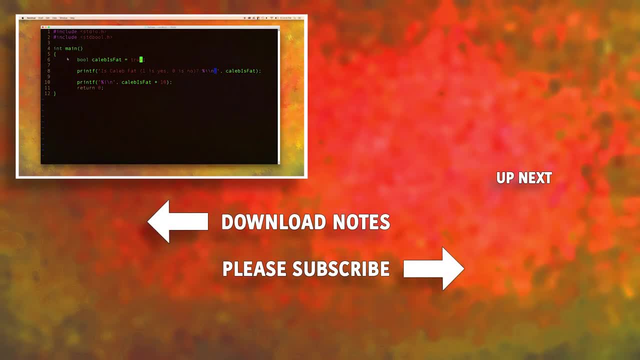 of the variable, but for now this is very good and i think this gets the point across of how boolean data works and how to use it in your program. so hopefully that was helpful for you guys if you've engaging with me in a similar way online in some夫. 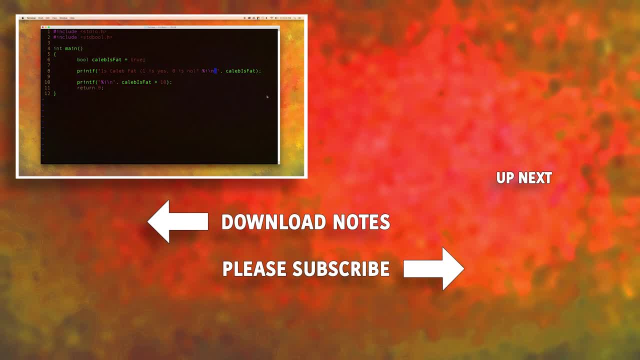 haf mor light, or, if you're dropikut correctly, i will goute this tutorialх. meanwhile, if you click the pause button, you'll see there is a littleotto say hi, maybe wanting toAcceptasthat sprawdkей'sdemeting and how to use it in your program. so hopefully that was helpful for you guys if you've been using our program. so 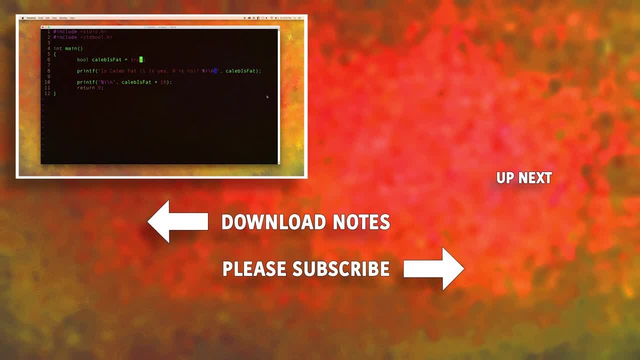 So hopefully that was helpful for you guys. If you've enjoyed it, please click like and click subscribe, as those two things very much help my channel. Thank you, guys, and I'll see you in the next video, where we will be talking about something new.